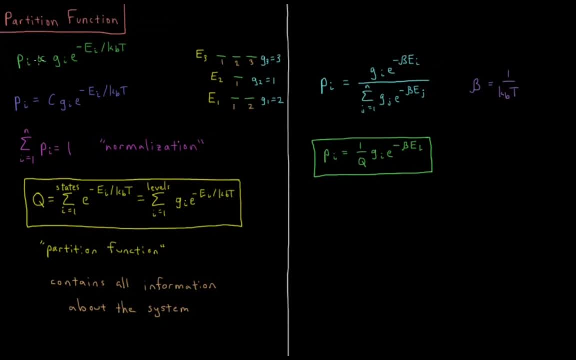 energy goes up. So since we have this proportional relationship here, that means there's some proportionality constant. so Pi equals C times Gi, the degeneracy times, the Boltzmann factor E to the minus Ei over kT. So the question now becomes: 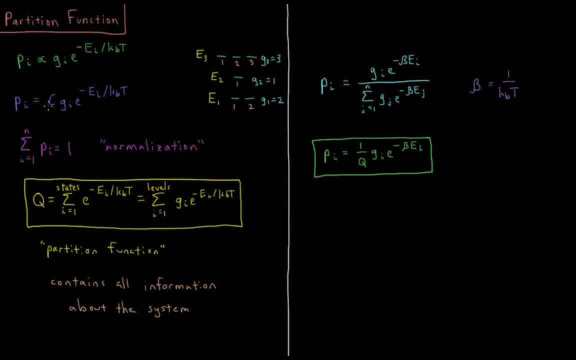 what's the probability of observing each of these states in our various systems? What is this proportionality factor? So how do we get our absolute probabilities of each individual state? Well, one concept we can use here is the concept of probability normalization. So each of these probabilities is a fraction of what likelihood occurs in that state. So 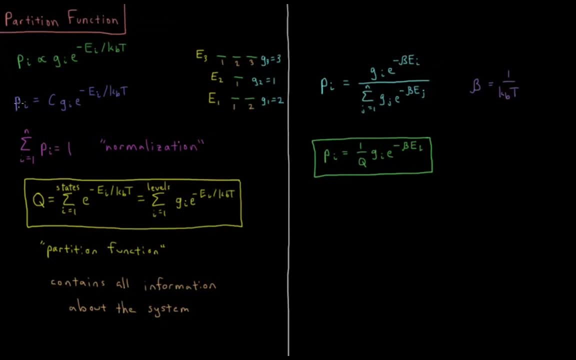 all the probabilities together should sum up to 100% or 1, that there's a 100% chance that the system is in a certain state. So the sum from energy level equals 1 all the way up to n energy levels of the probability of each energy level should equal 1.. There's a 100%. 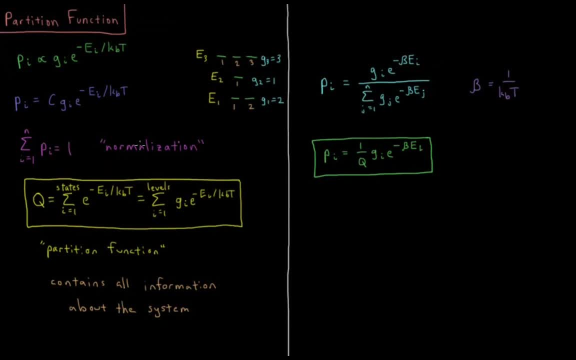 chance that the system is in some energy level, and that's called normalization. What we're going to define here is a quantity called Q, which we're going to call the partition function. So Q is a sum over all of the states of their Boltzmann factors. so e to the minus, ei over kt. 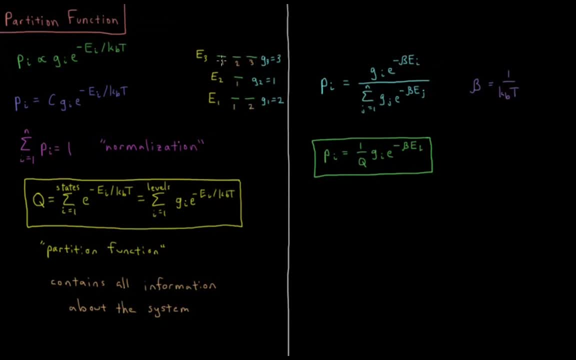 so states, here being all the each individual green bar that I have labeled with the orange state label. So we could sum sum over states this way of the Boltzmann factor of every individual state. or we could sum over energy levels, where we have sum of from i equals one up over every. 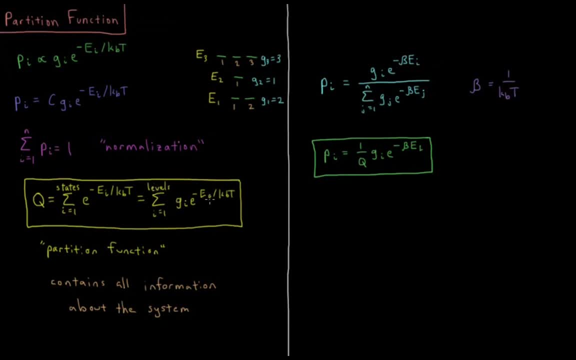 energy level of its degeneracy times, the Boltzmann factor of that energy level. So this is called the partition function and this contains all the information about the system. So it may not look like it now, but using this partition function we can. 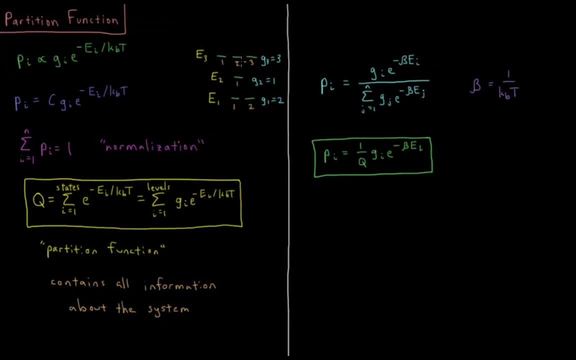 actually calculate every property of this system that there is to know. So if we have the exact partition function of a system, we can calculate the exact energy entropy, free energy, chemical potential, energy free energy, chemical potential, equilibrium constant- any quantity that you want to know about a system.